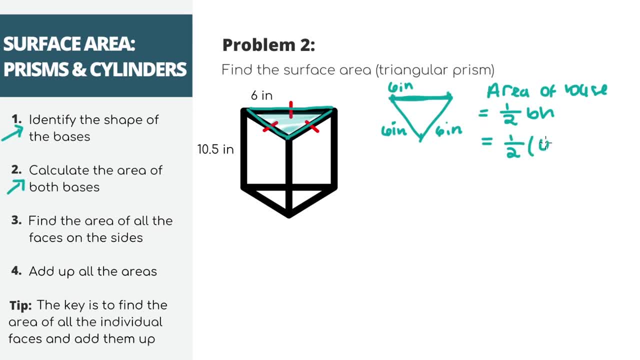 We have the base, which is six inches, but we don't have the height directly, So we have to use a little a squared plus b squared equals c squared action to find the height. first, Plugging in all the numbers, we're trying to find a. b equals three, since this is half of six and c is six. 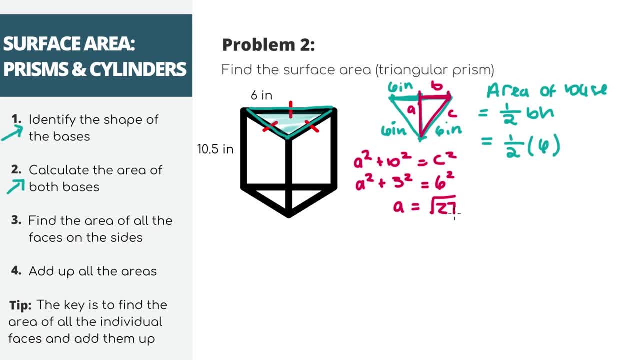 Solving for a, we'll get that the height is the square root of 27.. Finally, we can calculate what we initially set out to do, which is to find the area of the base. Let's plug everything into the formula one: half base times height. 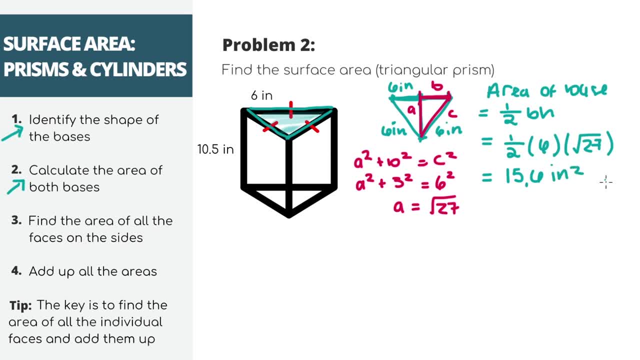 and we'll get roughly 15.6 inches squared. This is just the area of one base, and since there are two bases, let's double that. So the area of both bases is about 31.2 inches squared. Next let's find the area of the other faces on the 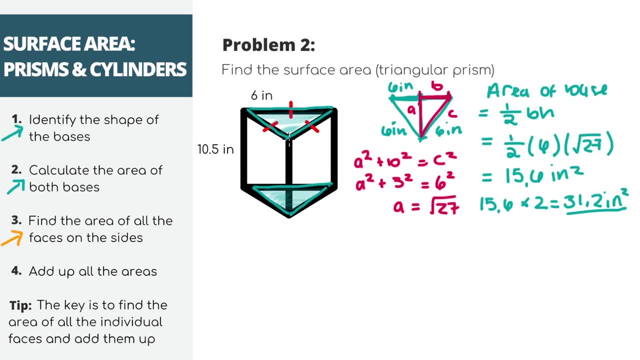 prism And these are usually just rectangles. If we look at this face, it's a rectangle and we can find the area of this one face as base times height. So six times 10.5, which is 63 inches squared. 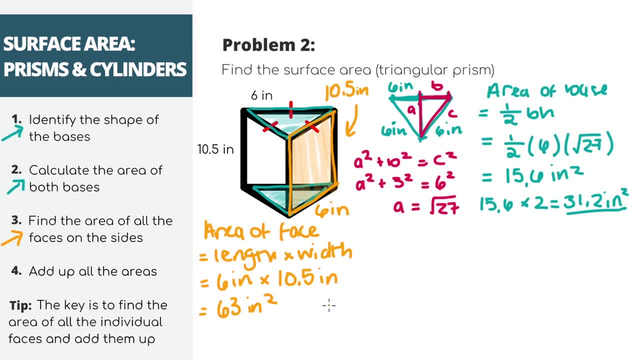 Now this is only the area of one face and we have a total of one to three identical faces. Remember there's one in the back. Taking 63 times three faces, we'll get a surface area of 189 inches squared for all of the faces on the side. 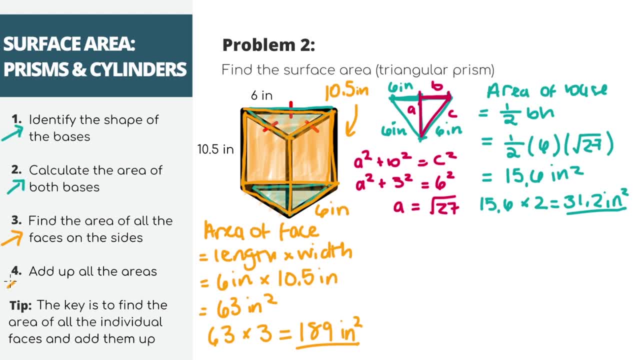 Finally, we've done all the hard stuff. Let's add them together to get the total surface area. We'll get eliminated if we don't find the box. Let's save the box for after that. Well, now there's four faces. it's wooden now. 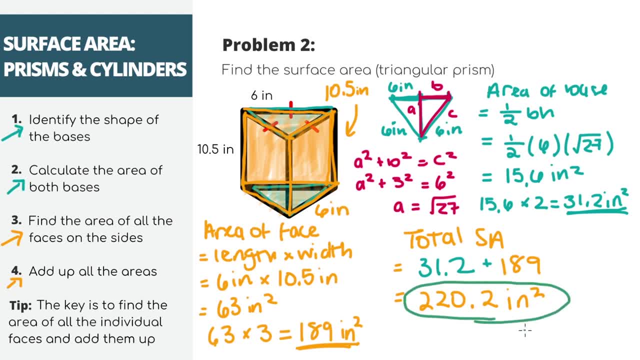 So we can just ignore both faces and scratch them off. Now, when you build a 71 mm old budgeted cell platform and weigh the number of PCNs, we have 220.2 inches squared. That's it. That's our answer. 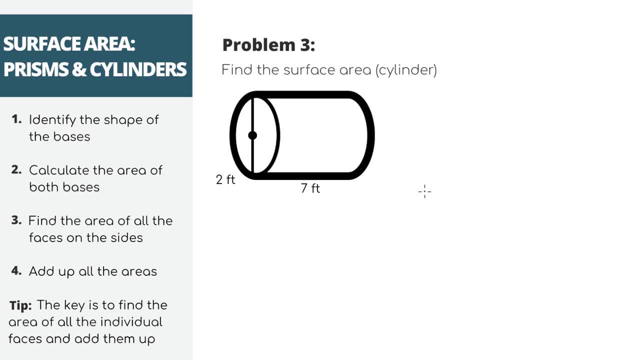 Next problem: we have a cylinder and it looks a little different than your typical prism, but the same steps still apply. Looking at the shape of the base, The bases are just circles. If you think of it, a can of soup is a cylinder, a roll of paper towels is a cylinder, and if you look 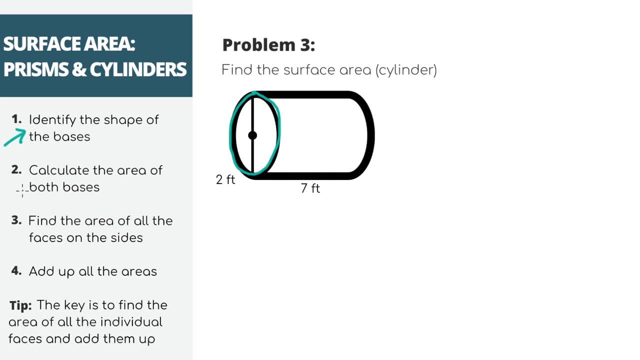 If you think of it, a can of soup is a cylinder, a roll of paper towels is a cylinder, and if you look at it from the top, the base, the base, toda, on your^^ bases are circles. To find the area of the base, the formula for the area of a. 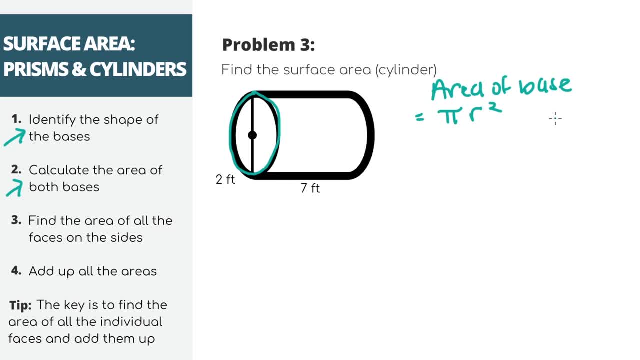 circle is pi r squared. From the diagram we're getting that the diameter is 2 feet. so we know the radius is 1 foot because the radius is just 1 half of the diameter. Plugging into the formula we'll get about 3.14 feet squared for the area. 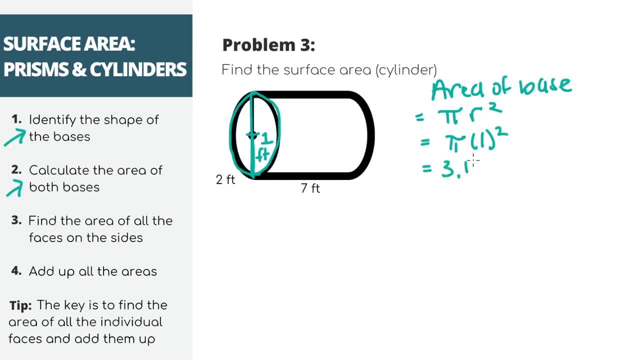 of one base. Let's double it to find the area of both bases and we'll get 6.28 feet squared. Our next step is a little different than what we've been doing, because it's a cylinder. it doesn't have all of these little individual. 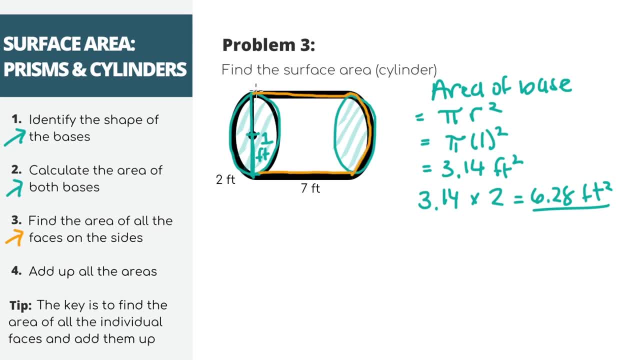 faces for us to calculate and add up. Instead, we're going to add up the area of one base and we're going to find the area of 2.28 feet squared. Instead, it's like this: one continuous face. If we think about a paper towel roll, that's a cylinder, let's think of the outside face. 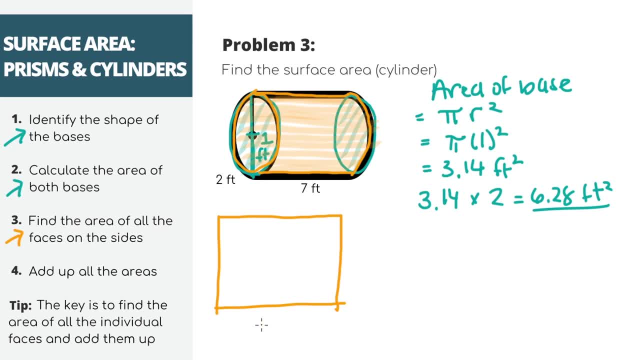 as one of the paper towels. If you unravel one sheet of a paper towel, it's just a rectangle, right For the dimensions. we know that the length of the paper towel is 7 feet. That doesn't change, And the height of the paper towel is the circumference of the circle. 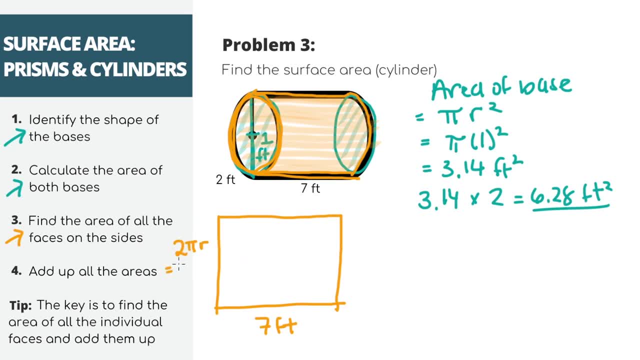 The formula for the circumference is 2 pi r and we found the radius earlier, so the height is 6.28 feet. Going back to what we originally set out to do, which is find the area of this paper towel rectangle, we're going to multiply the base times height. 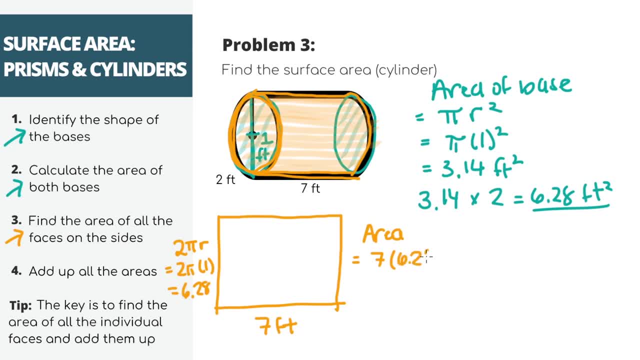 So 7 times 6.28.. And we're going to get an area of 44 feet squared. For our final formula we need the radius of the circle step. we can add up the areas 6.3 plus 44 and get 50.3 feet squared. That's it. 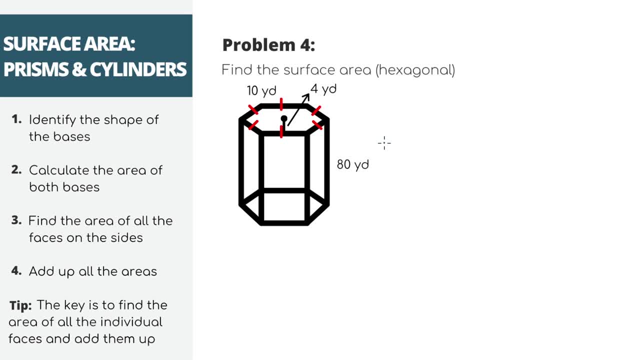 Last challenge problem. This is a hexagonal, hex, hexagonal prism. Well, the shape of the base is a hexagon where all six sides are 10 yards And this little length from the center to one of the sides is four yards If I redraw it from the 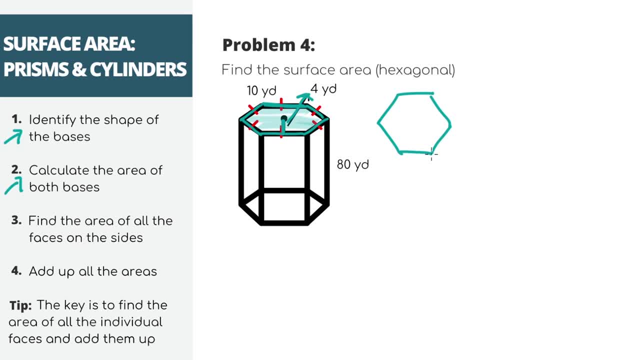 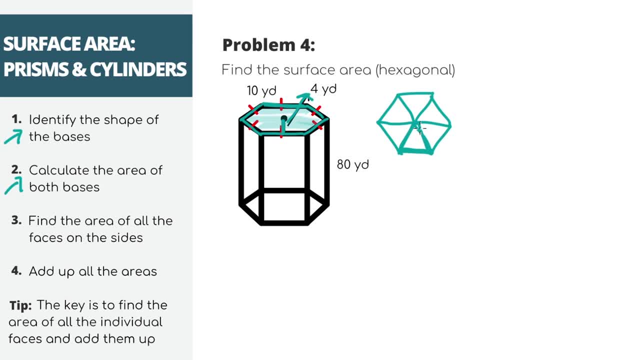 we can multiply it by six to get the area of the entire hexagon. Okay, the area of a triangle is one half base times height, So one half 10 times four, This equals 20.. Then, because there's six of these little triangles in a hexagon, let's multiply it by six. 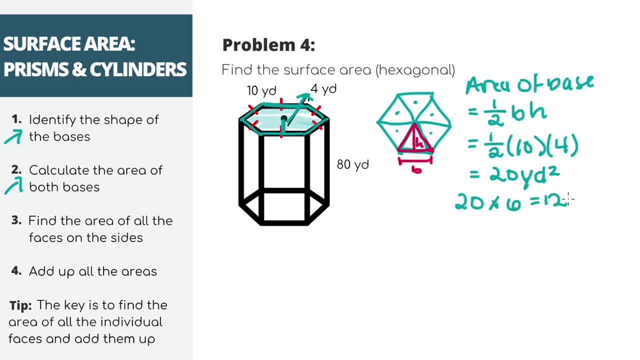 Then, because there's six of these little triangles in a hexagon, let's multiply it by six And we'll get the total area of this one hexagon is 120 yards squared. But because there are two bases, one at the top, one at the bottom, 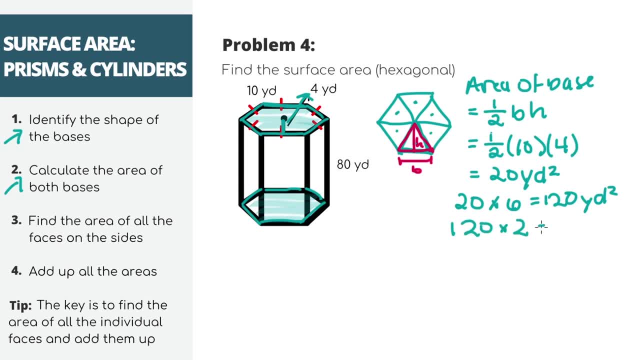 let's multiply by two And we'll get an area of 240 yards squared for both of our bases. Now finding the area of the outside faces: if we just look at one face it's a rectangle. So base times height, which is 10 times 80, is 800 yards squared. 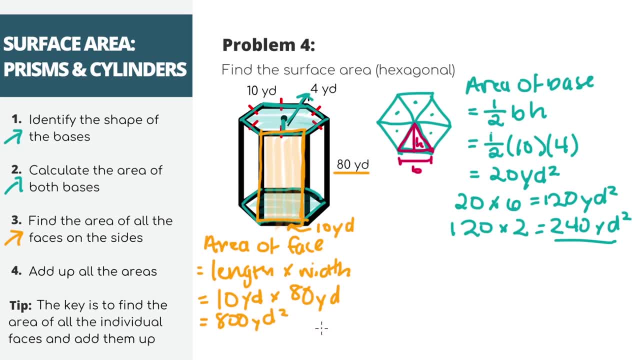 And there are a total of six faces. so 800 times 6 equals 4,800 yards squared. This is the area of all of the outside faces on the side In our final step of this problem and the final step of this problem.